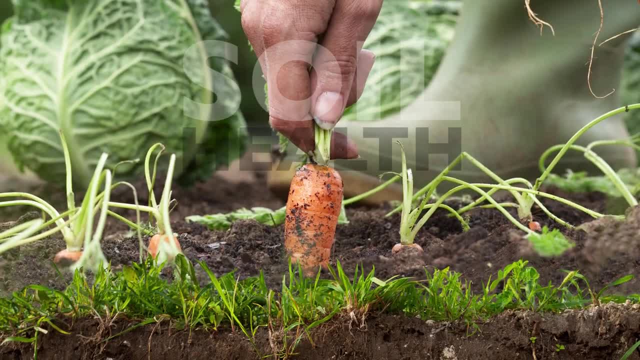 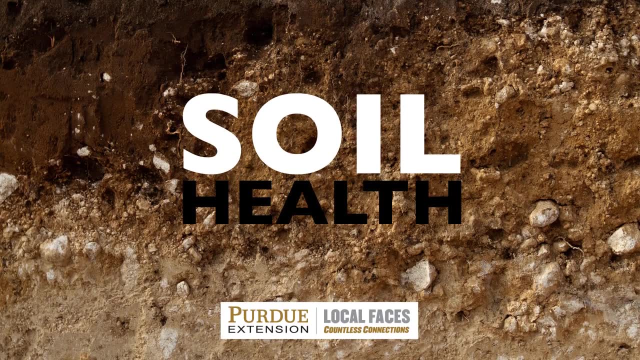 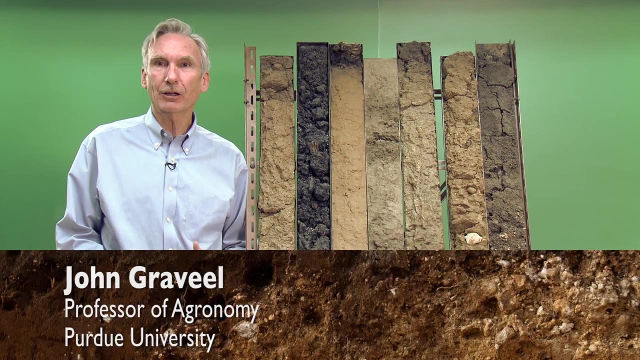 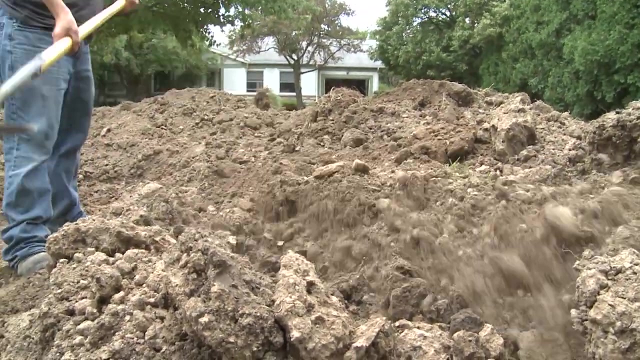 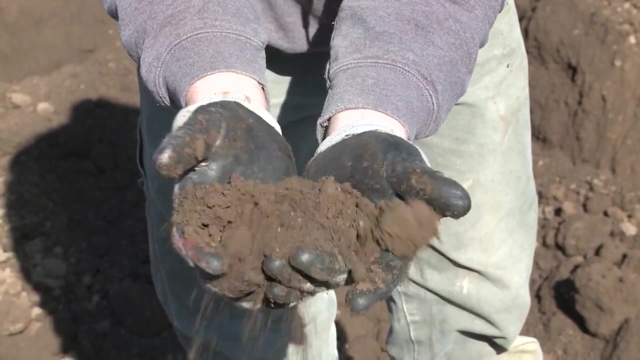 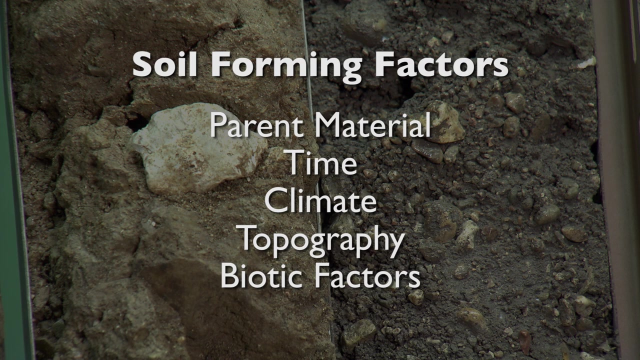 What we're going to do today is talk about soil origins and the formation of soils. Unconsolidated material which sits on the surface of the earth is actually impacted by five soil forming factors: Parent material, time, climate, topography and native vegetation are biotic factors. So what we are going 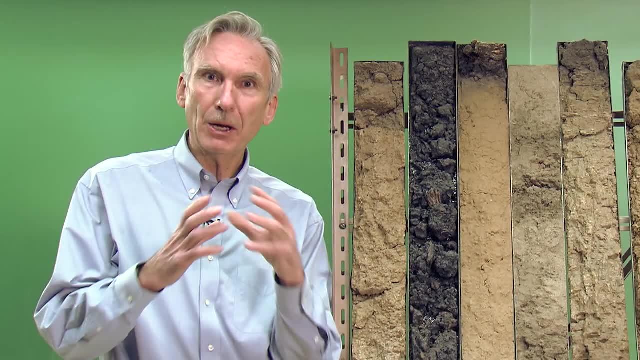 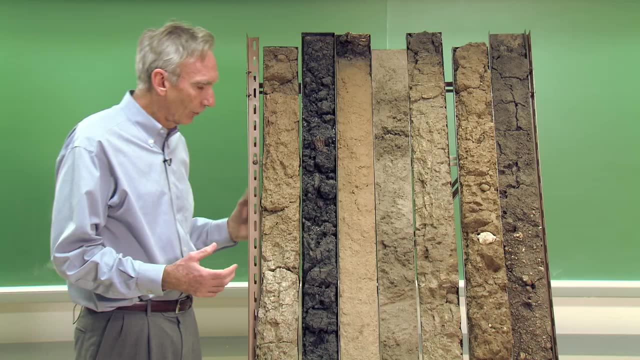 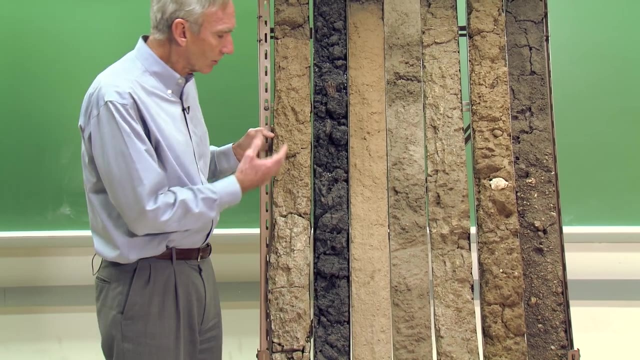 to do is focus in on just parent materials and show you the different parent material types that we have here in the state of Indiana. So the first monolith that we have here is a monolith with shale down here at the very bottom, And this soil has actually developed from that shaley type of 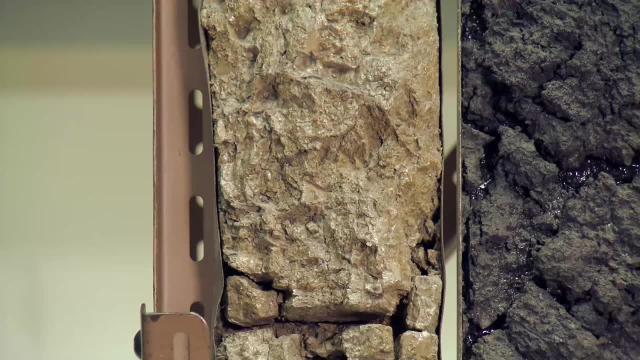 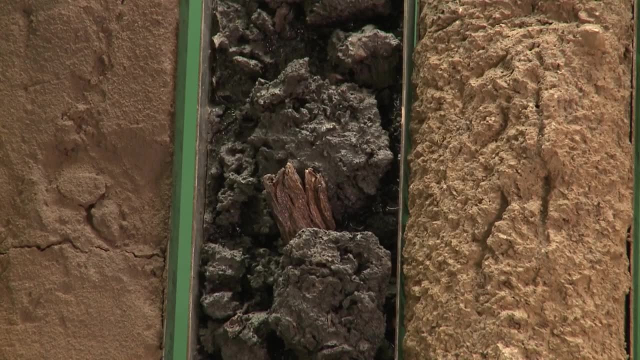 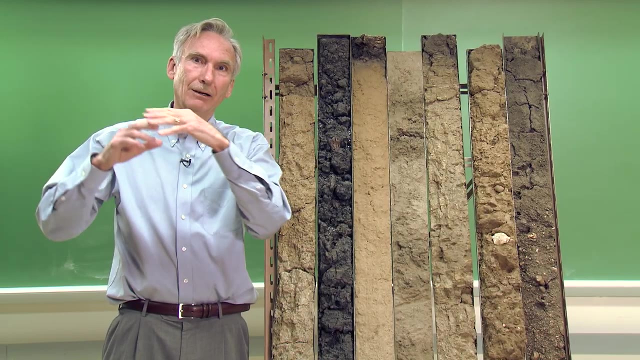 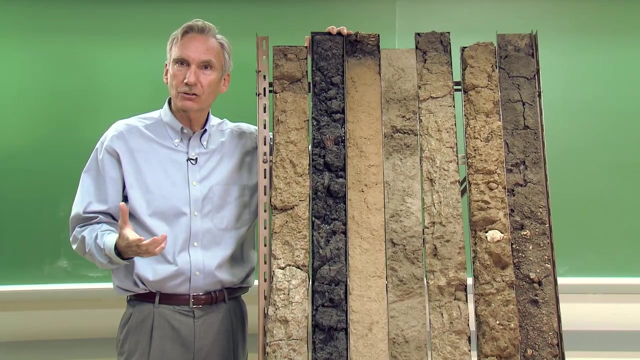 parent material. So this material is actually referred to as residuum, a residual parent material. One percent of our soils worldwide are considered to be organic soils. If you're up in northern Indiana, maybe in Michigan or in Wisconsin, what you'll find is that you will find pockets of organic soils In 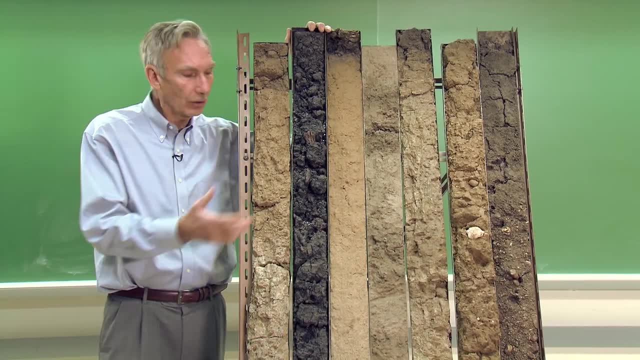 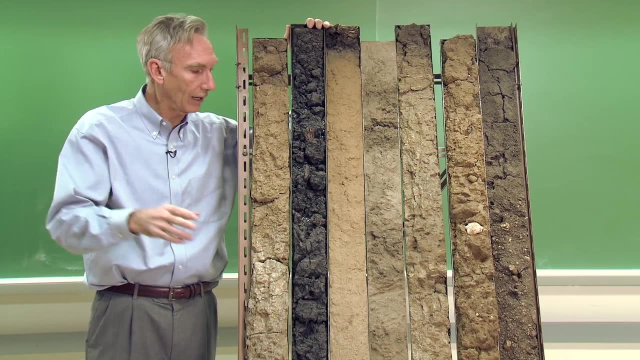 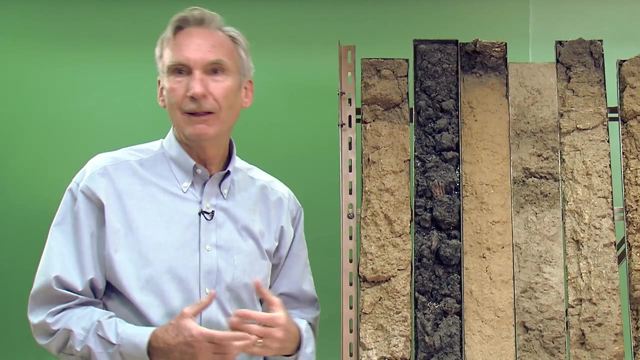 this particular soil. it's an organic soil because it has greater than 30% organic matter. So anything with greater than 30% organic matter is considered an organic soil. So the highest organic matter content you usually find in a mineral soil is somewhere between five and six percent organic matter, or seven. 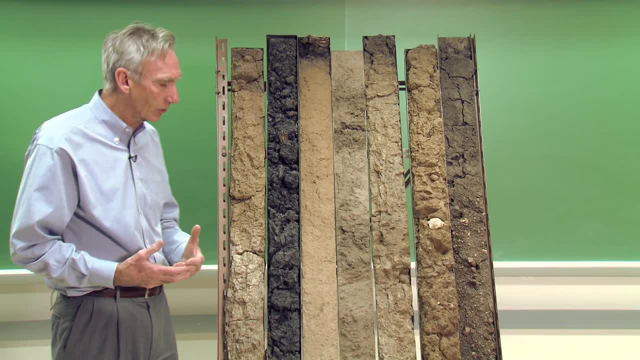 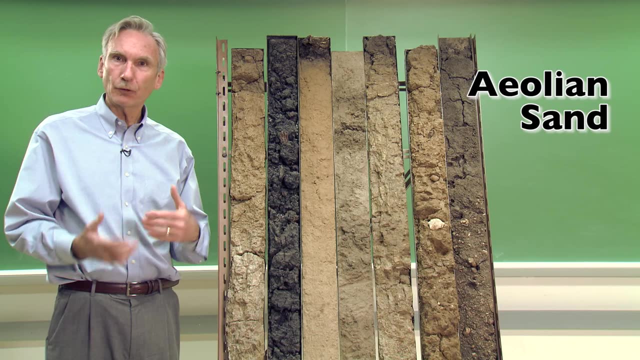 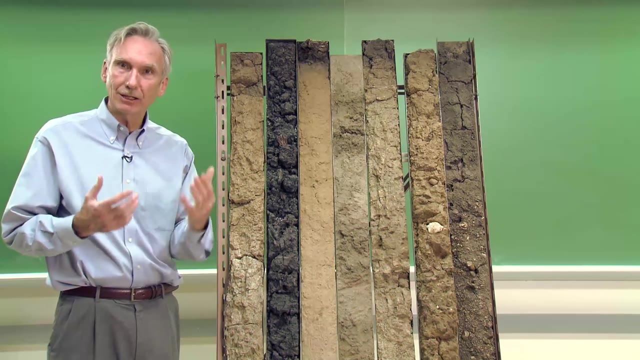 percent organic matter. The next type of parent material that we have here in the state of Indiana is called Aeolian sand. Now remember, in our first lessons we talked about the horizons in the soil. We talked about the A horizon, the E horizon, the alluvial. 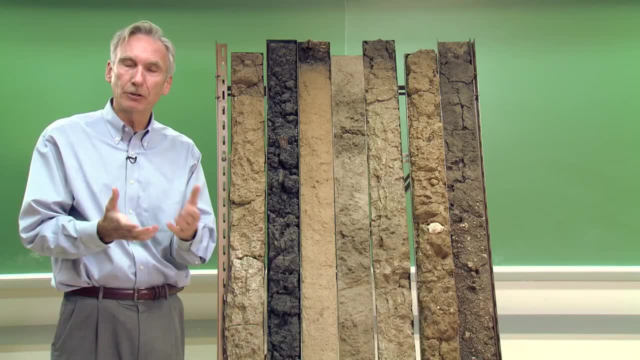 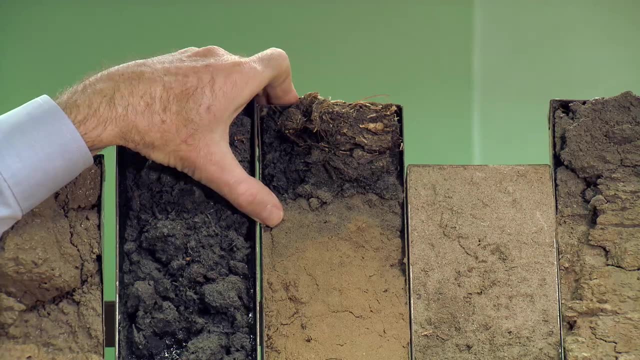 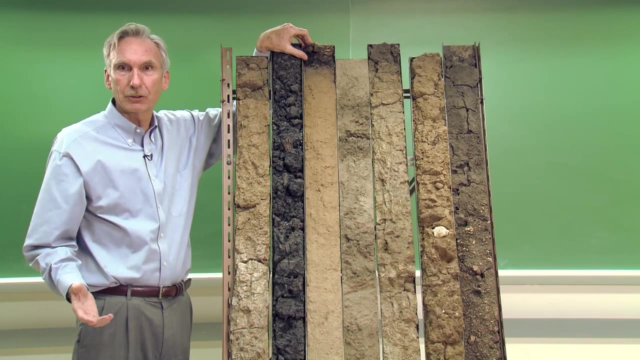 horizon, the B horizon, where everything washes into the B horizon, and the C horizon, which is the parent material. Well, in this particular case, you've got the A horizon right here at the very top, and the rest of this is C horizon material or parent material, And so 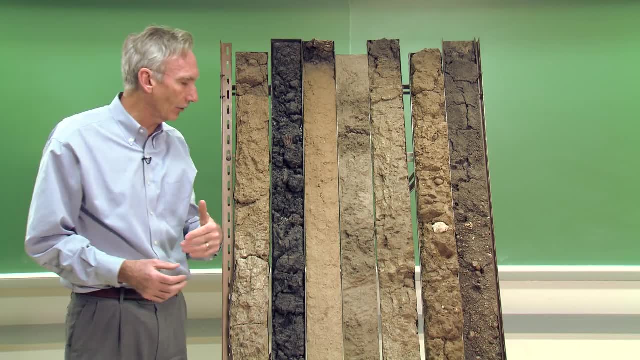 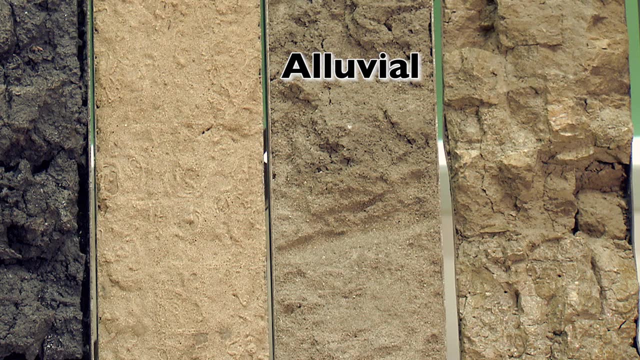 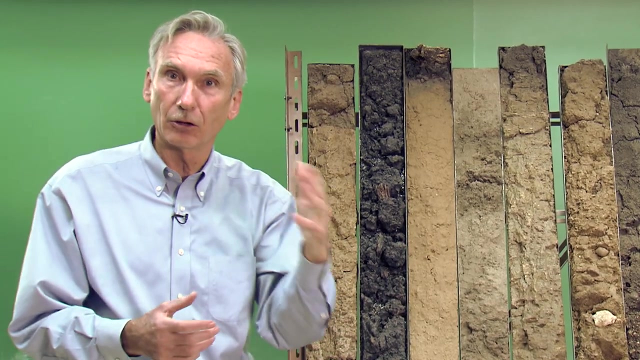 what's happened is that wind has blown dune sand along, and so what you get is these Aeolian deposits of sand. This is called an alluvial soil, a very common feature that we find here in Indiana along major rivers like the Wabash River. 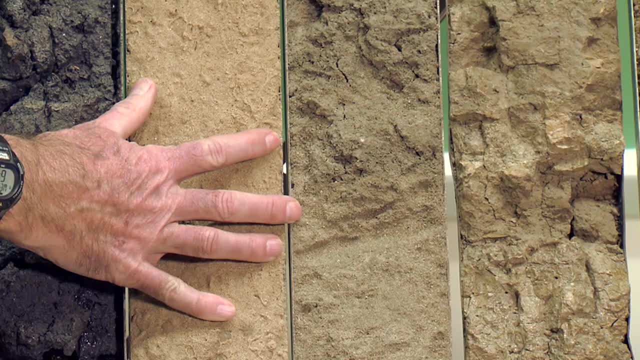 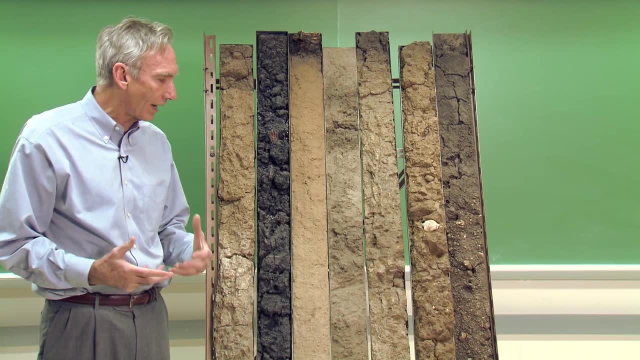 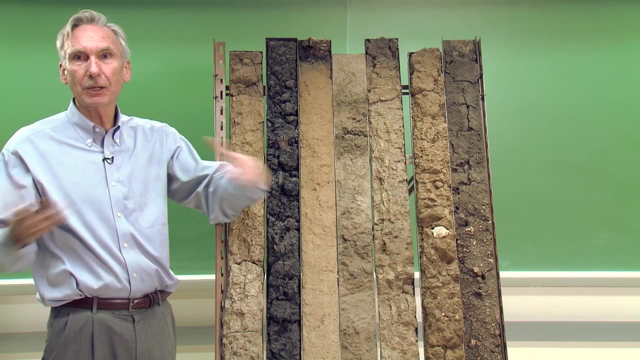 the Tippecanoe River, the White River, and here's a black layer in this, in this profile, here And in that back black layer. what's happened is that the plants have developed. flood came along. this water is sitting on top of those plants. the plants die alright and contribute. so this black zone to the 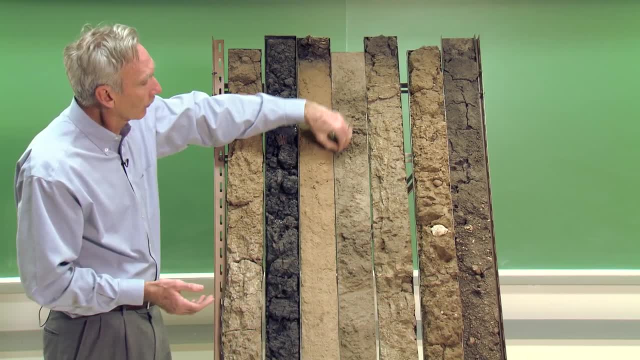 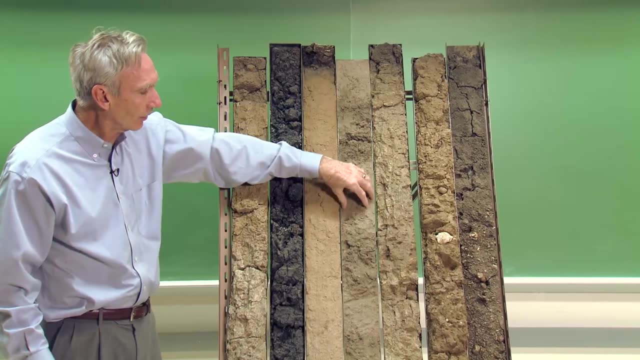 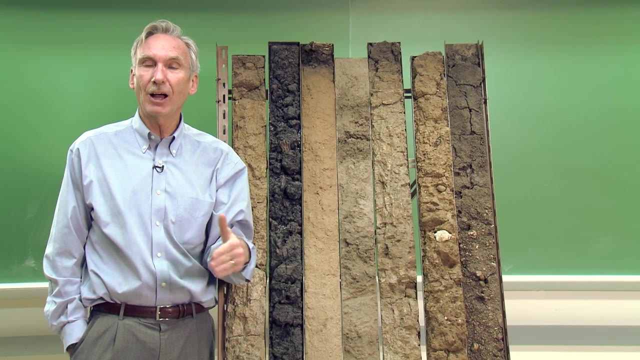 soil And then what happens is that you get reestablishment of plants again, the plants grow and then you get another flood the next year. So these soils here, these alluvial soils- this is where you're going to find the youngest soils in the state of Indiana. 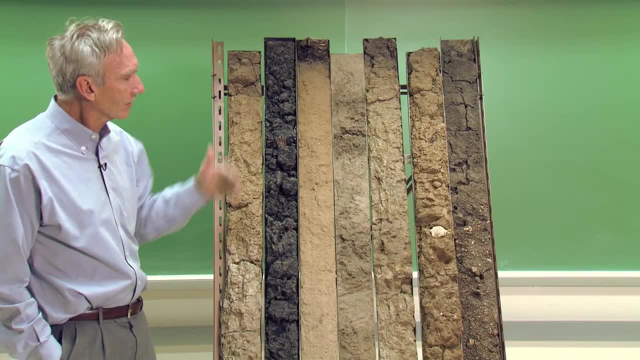 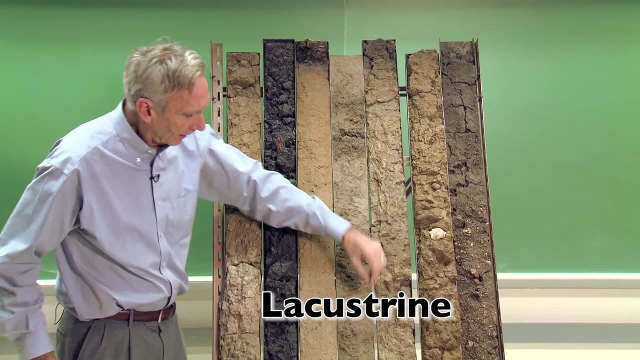 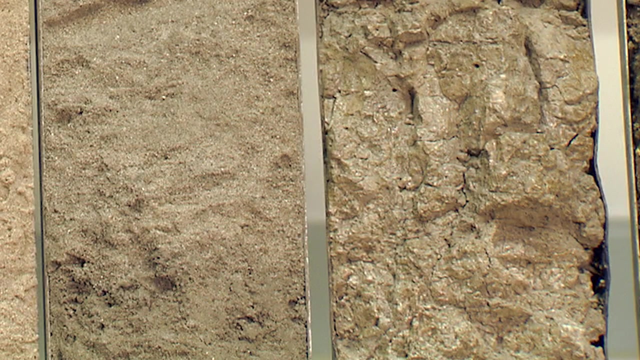 are found along the flood plains, alright. The next soil profile is unique as well. It is a Lacustrine parent material. in the Lacustrine parent material you get these bands that are kind of going across here down at the bottom, down in. 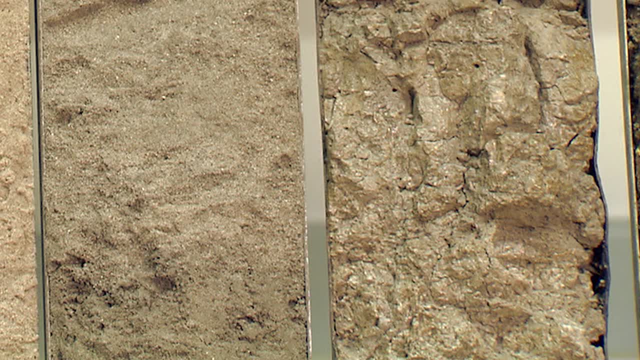 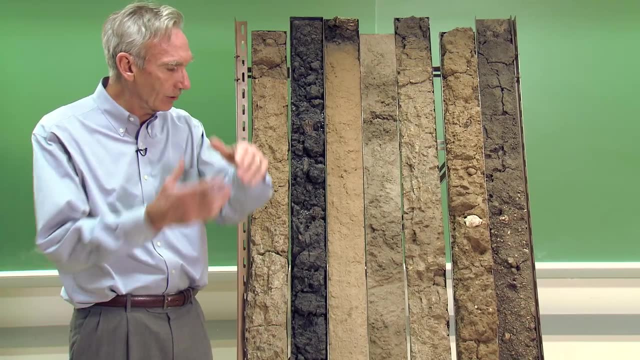 the C horizon, the parent material horizon, and in those those bands are layers of sand that you want to light up. you want to group them, make them in a of silts and clays, when this huge lake that used to cover part of the Fort Wayne area, 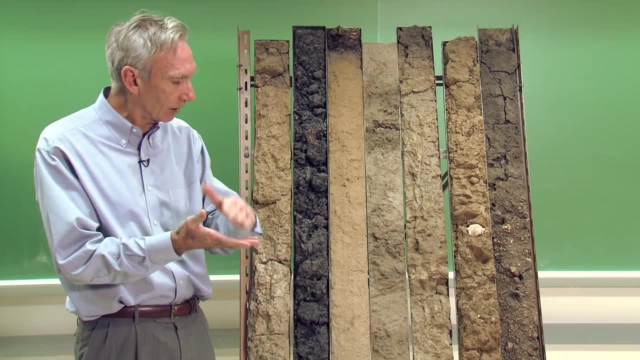 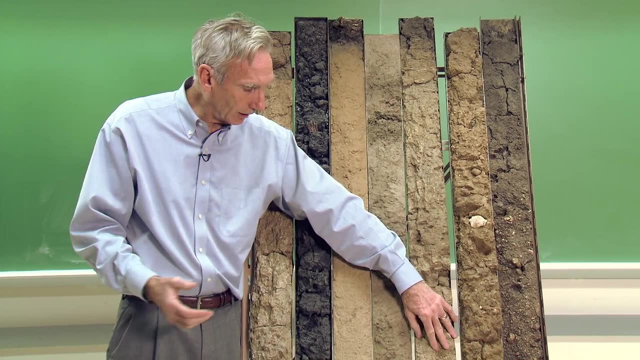 evaporated, and when it evaporated, lots of silts and clays settled out, And so what's unique about this particular soil? especially if you're a farmer in the eastern part of the state, in the Fort Wayne area, it's very difficult to pull a tillage. 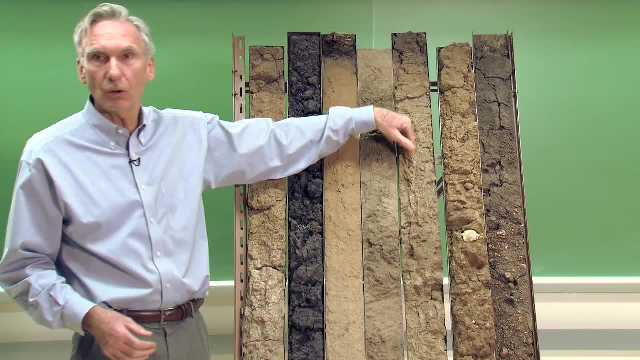 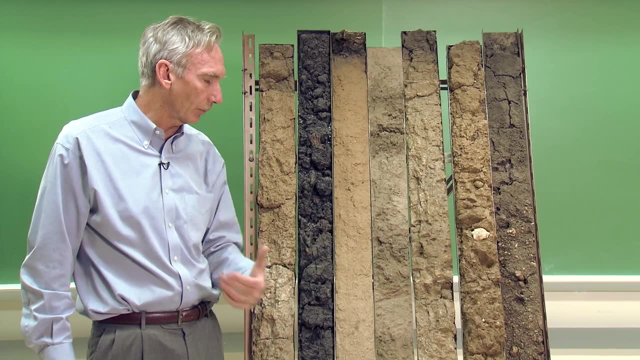 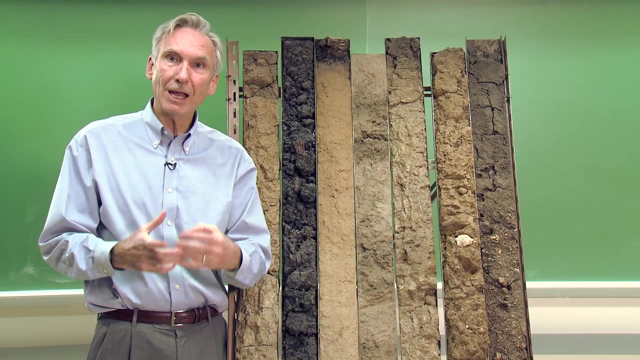 implement through something like this. This can be a productive soil, but at the same time, it's going to take a lot of energy, more energy, to actually pull a tillage implement through a soil like this. Now, the two most common types of parent material that we have in the Midwest are glacial till. 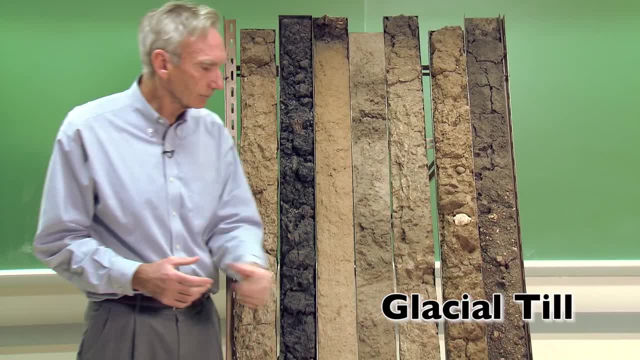 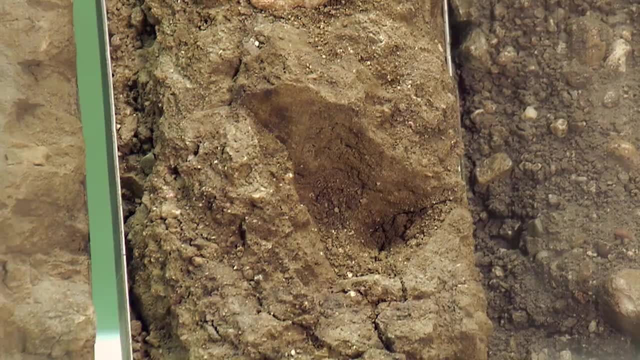 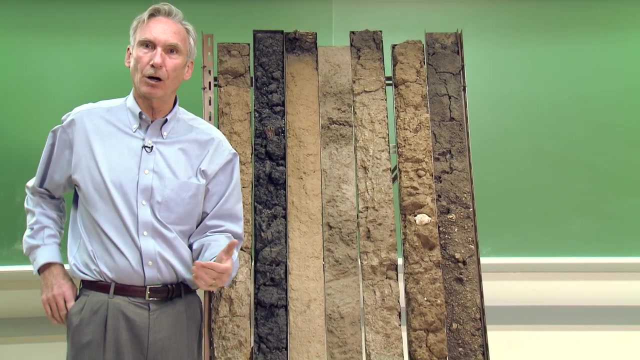 and glacial outwash. Glacial till actually consists of a compact parent material, So the rocks are very sharp. they're all mixed together with sand and clay and silt. everything's mixed together. that is glacial till, This soil. here the parent material is glacial outwash. 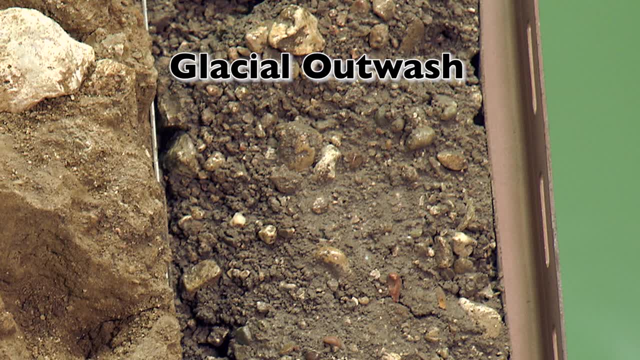 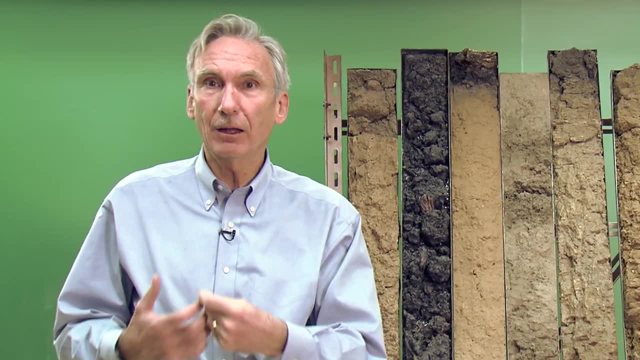 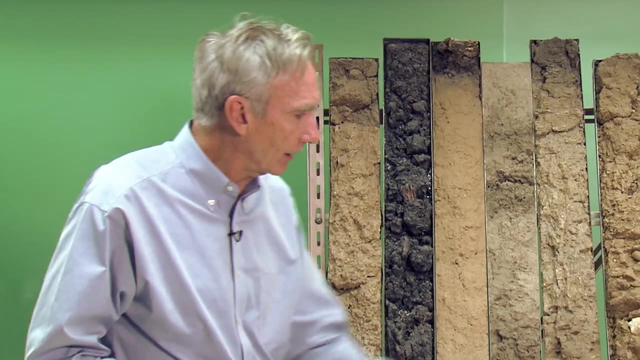 In glacial outwash. actually, the rocks are rounded, they're smooth This period of time when the glacier started to melt and what happened was there's this huge volume of water flowing down the river And what would happen is it would pick up some of these rocks and it would roll around. 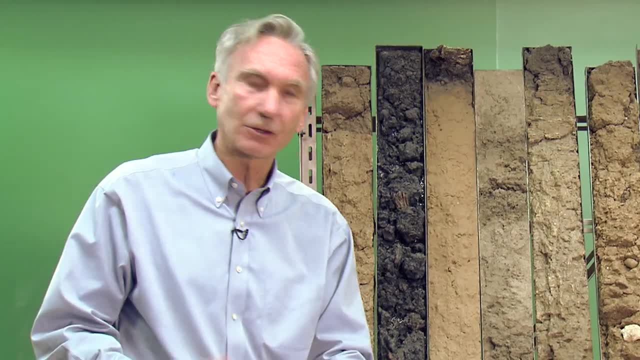 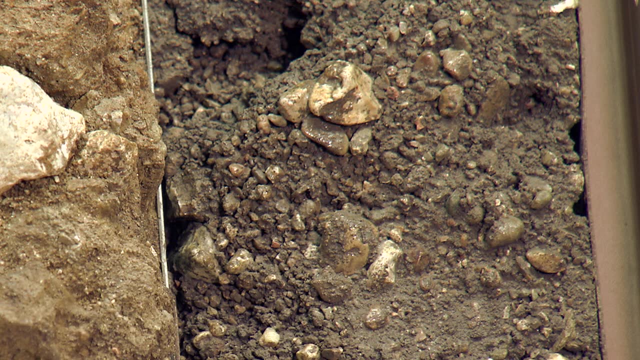 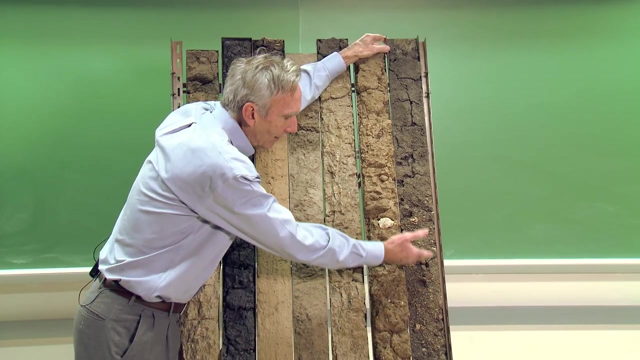 in the water and actually smooth off their surfaces, And so you get these very smooth rocks occurring in glacial outwash. Also, it's stratified, The drainage is excellent, So think about it. You've got these big pieces of rock down here. water just moves smoothly, quickly through. 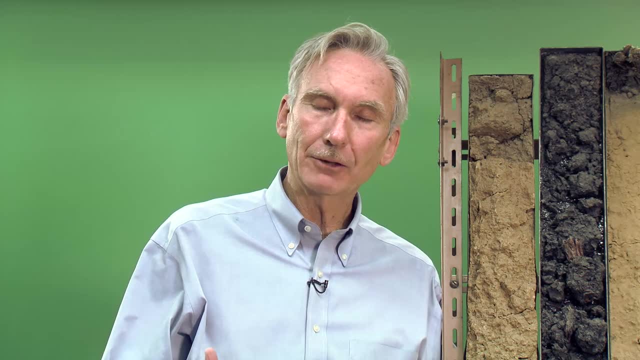 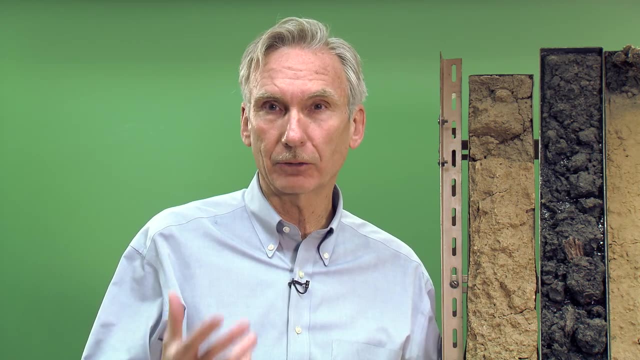 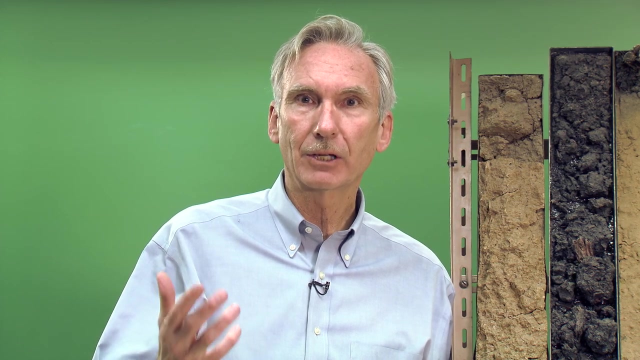 soils like this. So the final comment that I want to make about soil formation is that glaciers have played, have had a tremendous impact on soils here in the state of Indiana. So we've actually had three glacial periods: The Kansan, which was millions of years ago. 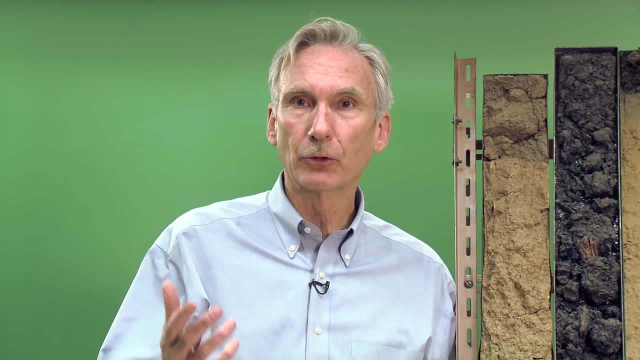 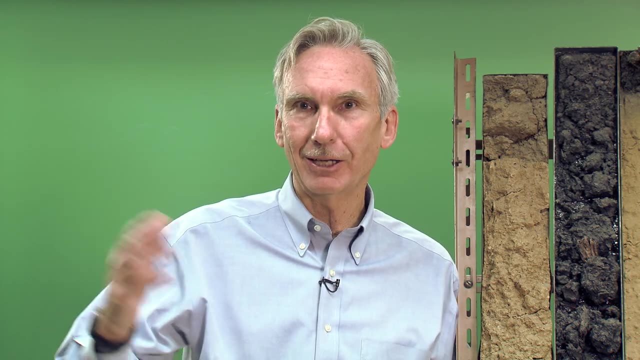 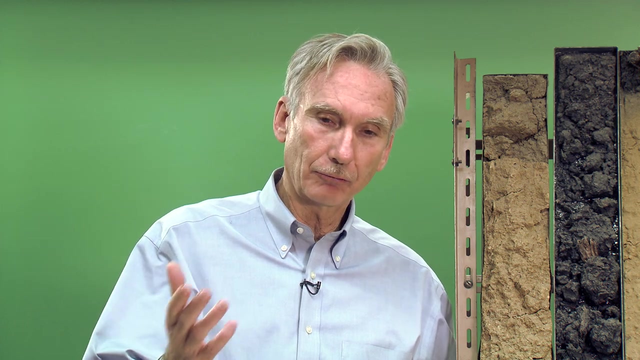 The Illinois, which was 200,000 years ago, And most recently the Wisconsin glacier, which has essentially moved out of the state of Indiana 15 to 20,000 years ago. So the soils in the northern part are actually from about Seymour, Indiana, which is a little. 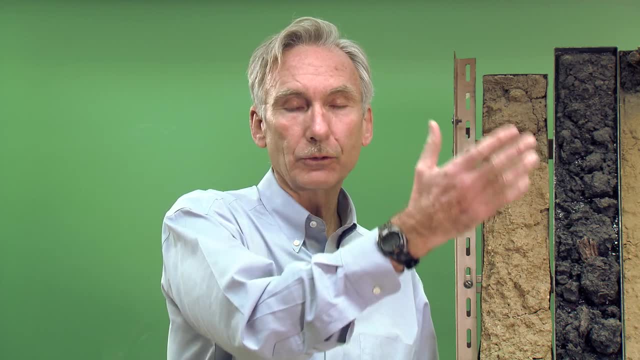 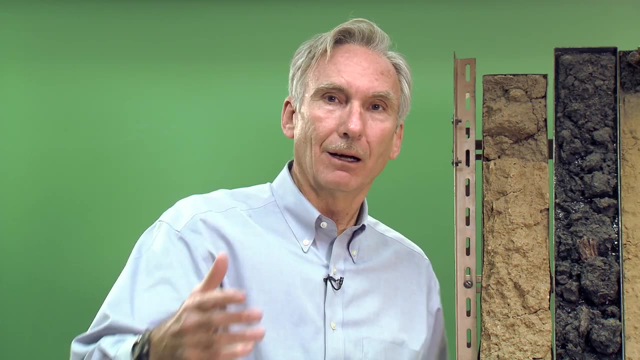 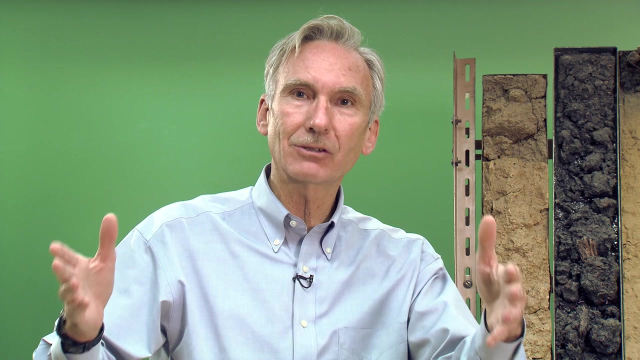 south of Indianapolis Northward. those soils were developed in Wisconsin. glacial material, The soils south of Seymour, Indiana and sort of wraps around the sides of Indiana. those soils were actually developed in Illinois and in Kansan. glacial material. 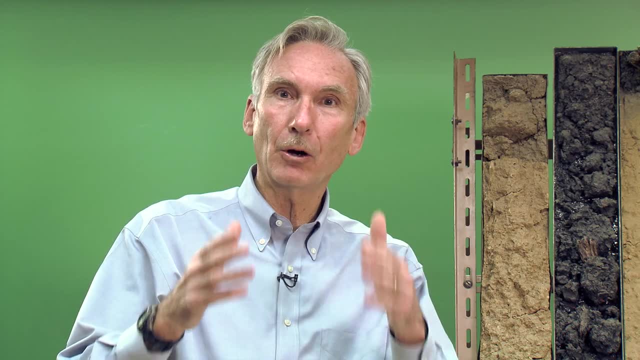 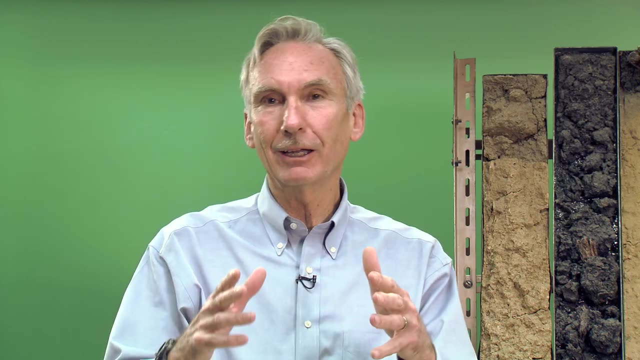 Interesting about the state of Indiana is that the south central part of the state was not glaciated, And so that's why the Bloomington area is so hilly. The glaciers had a tremendous impact on soil formation here in the state of Indiana.